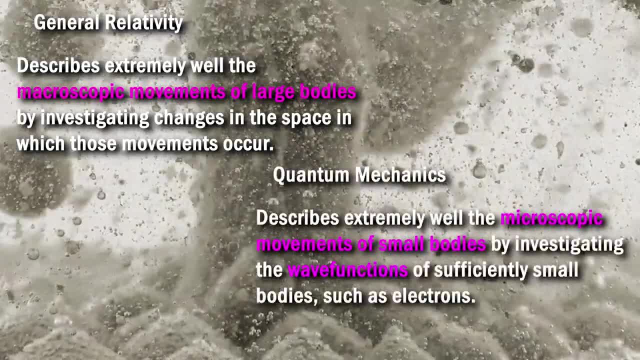 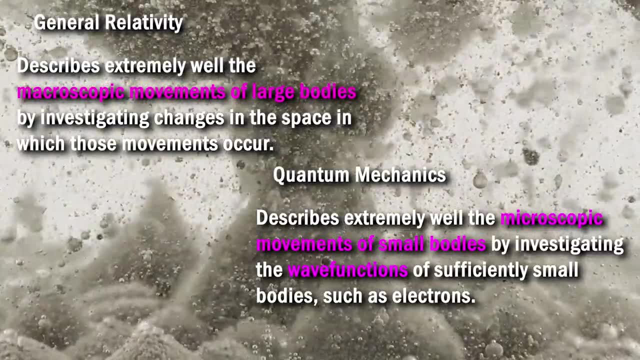 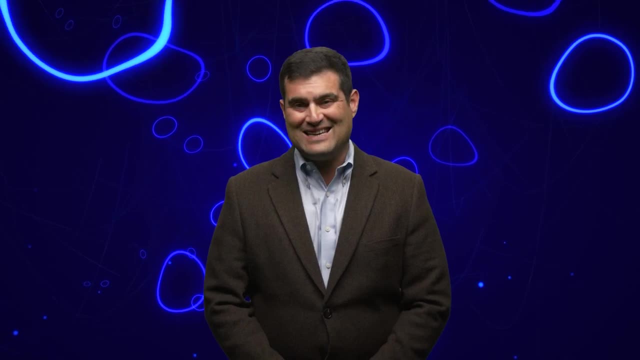 matter how to move. Quantum mechanics describes the behavior of subatomic particles, of the, on a framework far removed from our classical expertise, and so we can't use our intuition from, say, the equations of Maxwell or the equations of Isaac Newton, classical mechanics. nevertheless, quantum mechanics is our perhaps most best tested theory of the microscopic behavior of particles. 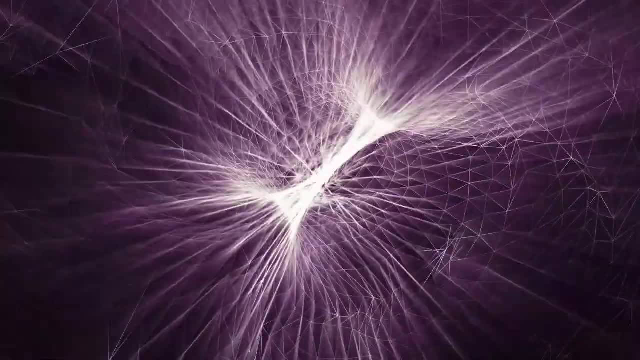 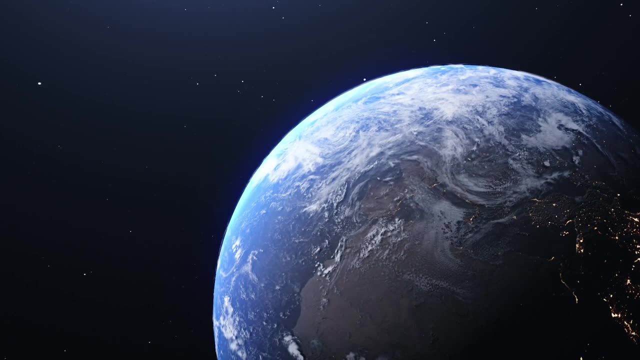 forces and fields. general relativity is our best description of gravity and we actually use it every time we use a GPS receiver. it computes gravitational general relativistic distortions that would otherwise lead us astray, and I always like to thank that, because I don't need more. 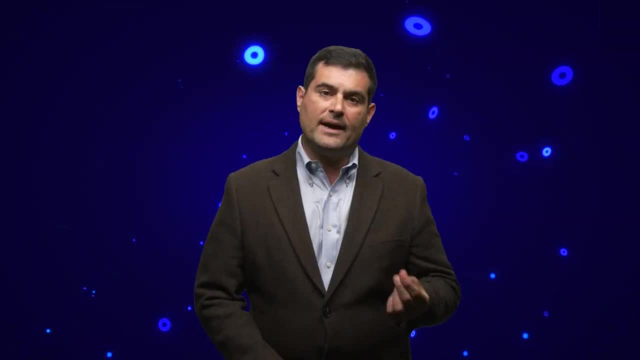 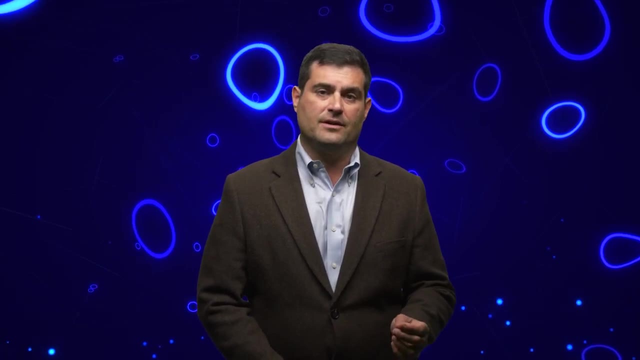 people yelling at me for getting off course in life. but the challenge of reconciling quantum mechanics, the very small, with the very large, of classical mechanics in general, relativity, which is a classical field theory, is about bridging the seemingly unbridgeable gap, and string theory comes. 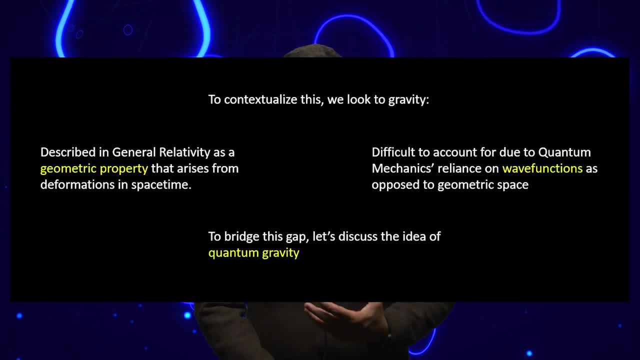 in there as well. the question is: can you make string theory emerge and also play nice with quantum mechanics as a way of formulating the origin of space and time, or the origin of space and time, and the origin of time and time, and space and time and time, and? 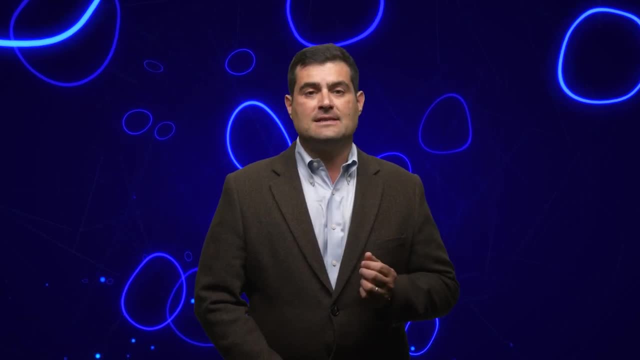 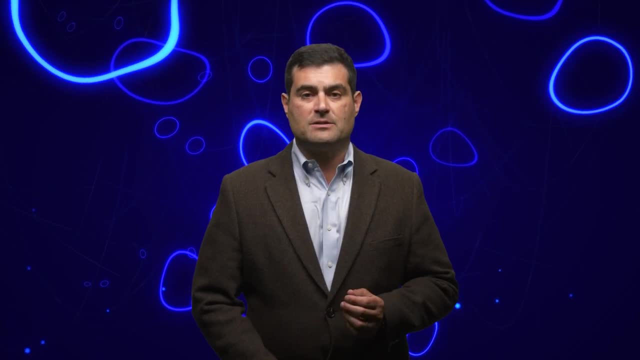 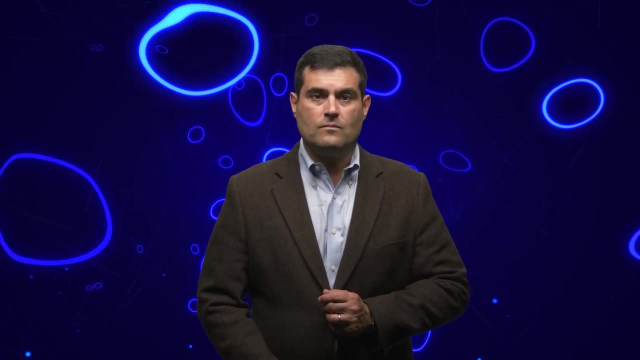 have been made against loop quantum gravity that it fails to meet certain experimental observations or even make new predictions. Nevertheless, we'll talk more about loop quantum gravity another time. So we understand gravity as the effect of curved space time. What curved space time? As I said, 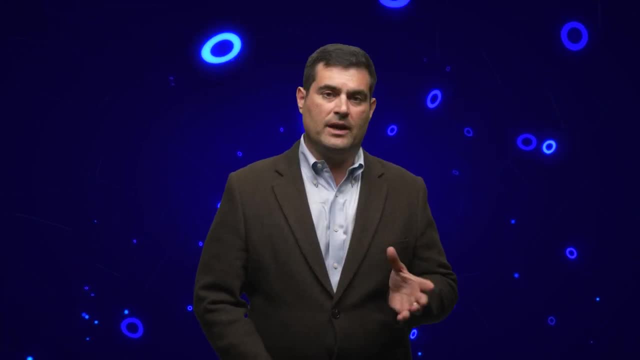 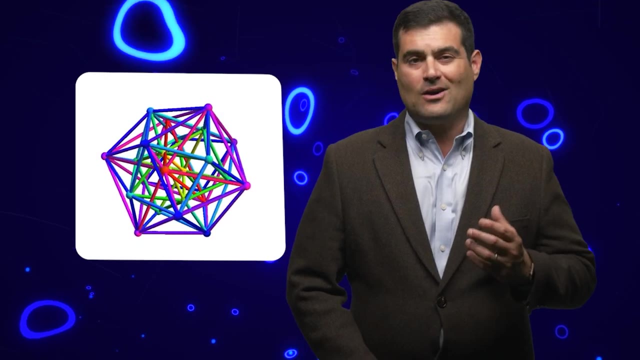 matter. So you have this interplay, this nonlinear behavior between gravity and the effects of gravity, of matter causing gravity and then being affected by gravity. So what can we glean about the quantum world which describes the behavior, trajectories, et cetera, and the future descriptions? 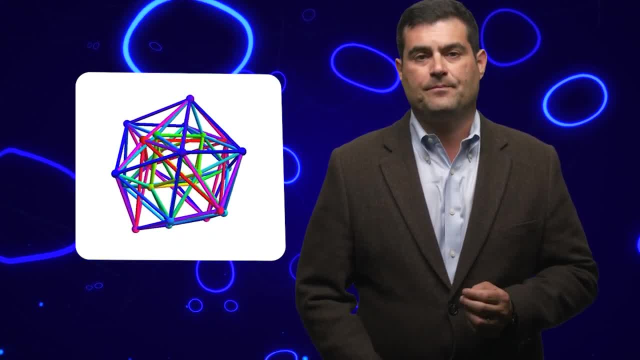 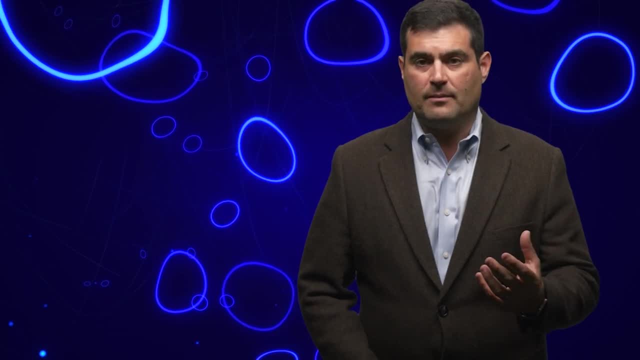 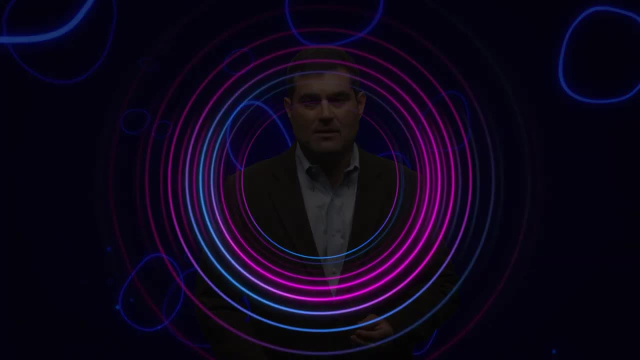 of subatomic particles via what are called wave functions. We can see the importance of string theory when we look at how the classical description of space, time and quantum mechanical processes break down when you have so-called ultraviolet Divergences. These are places where we're effectively dividing by zero. We have 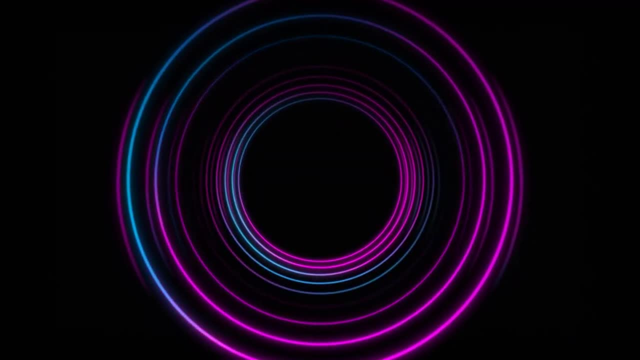 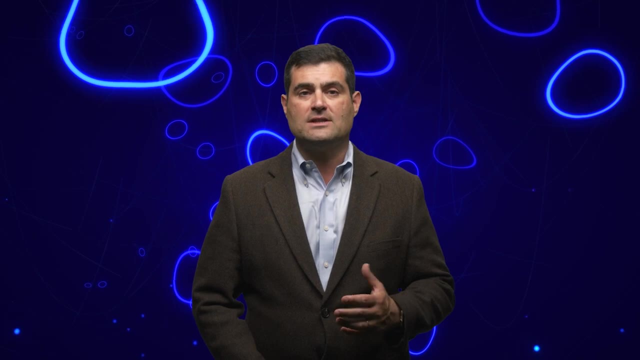 infinitesimally short distances, and we have macroscopic charges, forces and fields, And at those regions the behaviors obtain breakdowns, And so you'd like to have a nice smooth manifold rather than dealing with infinitesimal point particles. And we'll get to those manifolds in 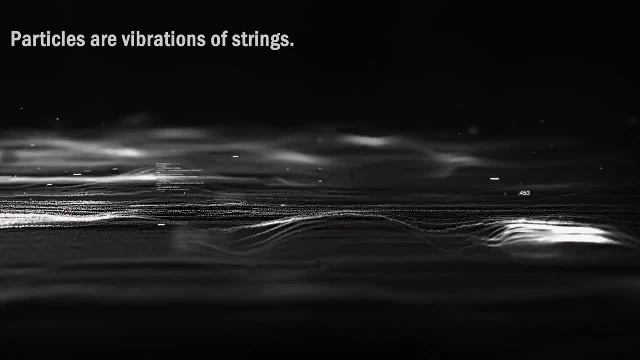 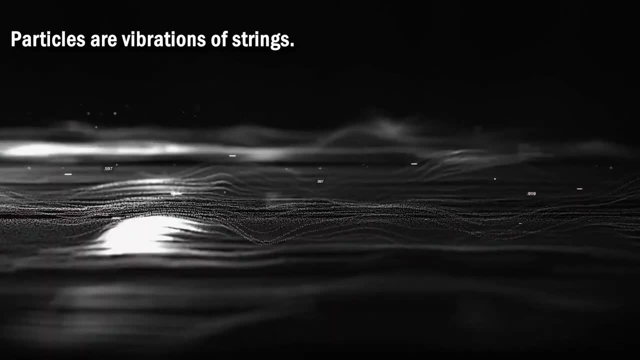 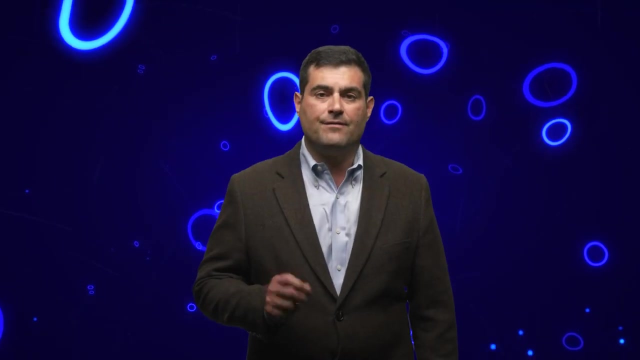 just a bit. What string theory fundamentally says is that particles are just multidimensional strings that vibrate like different notes plucked on a guitar string. When you play the right note, the strings can interact in different manifestations: They can be quarks, they can be photons, they can be gluons, electrons and all of the fundamental particles in 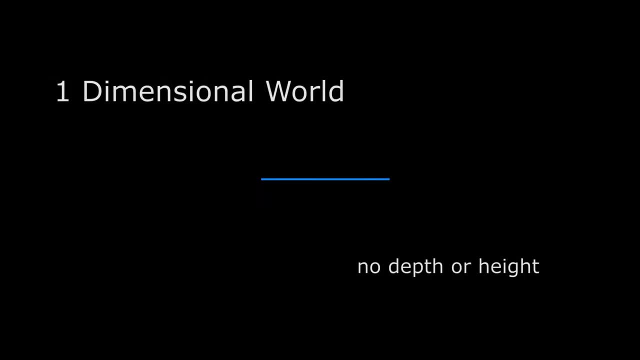 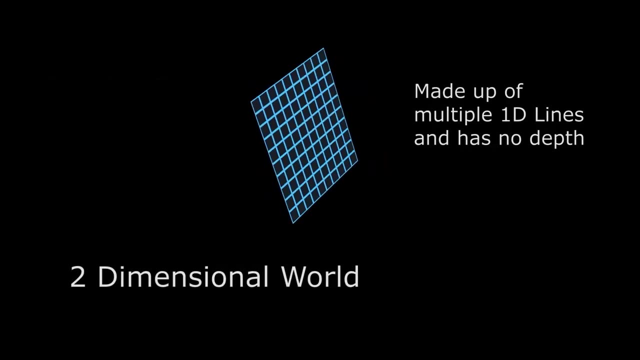 the standard model of particle physics. At small scales, though, these extra dimensions are hidden and we don't recognize them. So we have to look at them and see. why don't we see these extra dimensions, these dimensions beyond the familiar north, south, east, west and up and down the three? 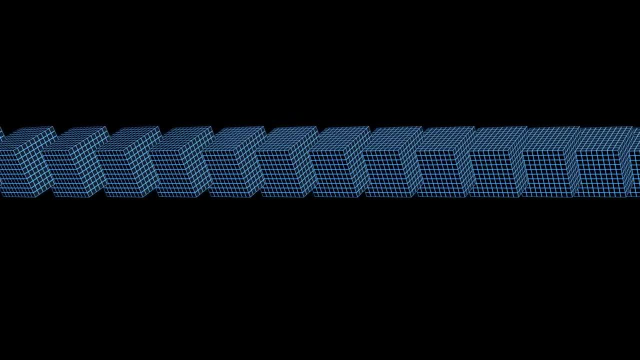 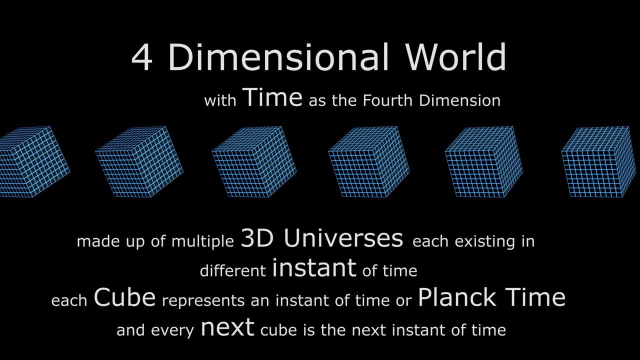 dimensions of space plus our one time dimension. So we actually may need many, many more. We don't have enough space time dimensions. But an analogy could be if you consider a bug: Imagine a bug and he's going to meet his friend for a little bite to eat. It happens to be a cookie on the floor. 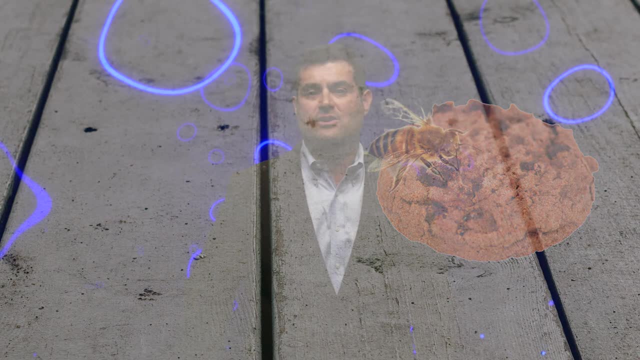 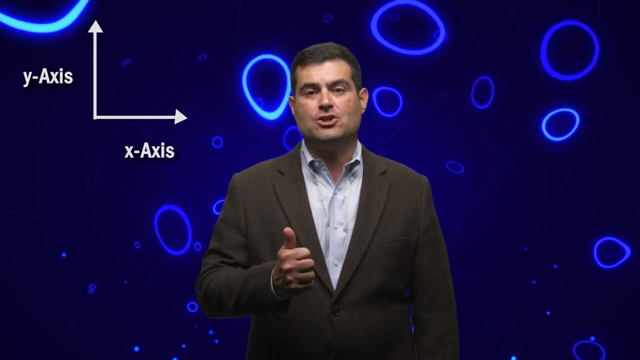 But if the bug only knows the X- Y coordinates of where that bug is on the two dimensional floor surface, his friend may miss the fact that the first bug is actually sitting on top of the cookie And in other words, in the third dimension, the two dimensional plane, the floor is essentially. 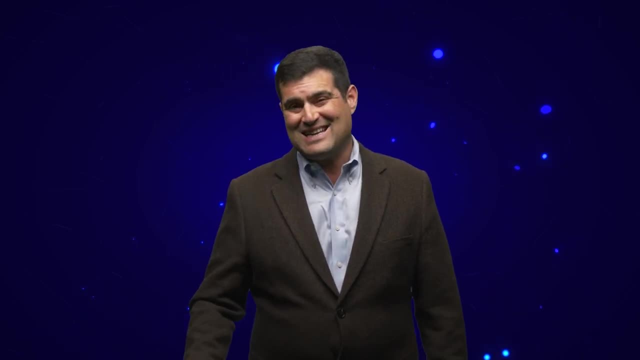 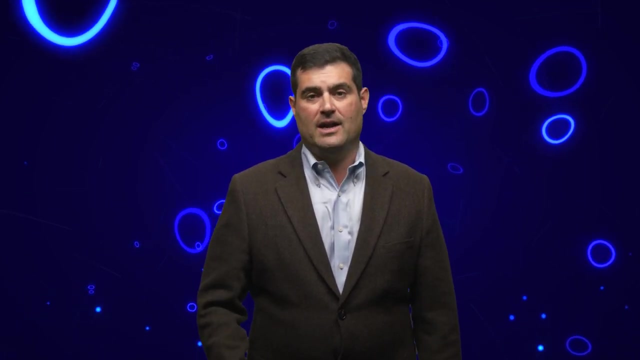 the projection of a three dimensional surface onto one lower dimension. It's not exactly compactifying, It's just a way of representing that you may need more than just the familiar dimensions that we operate in and that we are familiar with to describe the physical phenomena that are of 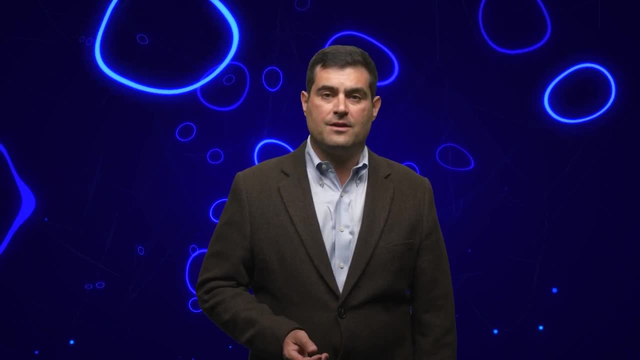 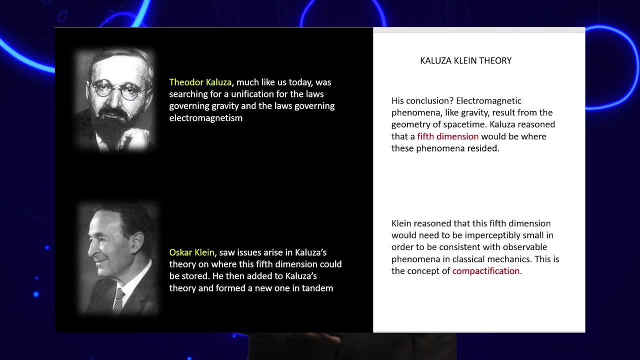 interest in this quantum theory of gravity. There actually was a theory that added to the dimensions of space and time an extra dimension, And this took place over almost 100 years ago, And it's known as Kaluza-Klein theory, And it's really the ancestor of string theory in a certain sense. 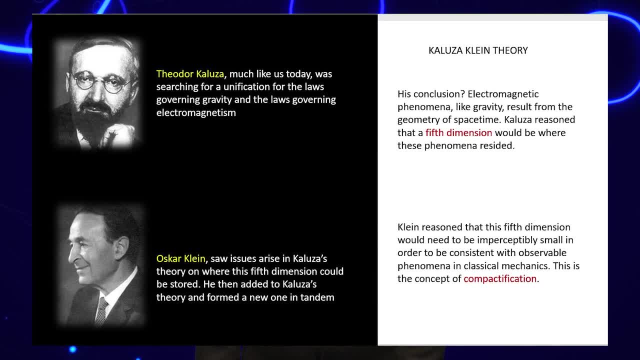 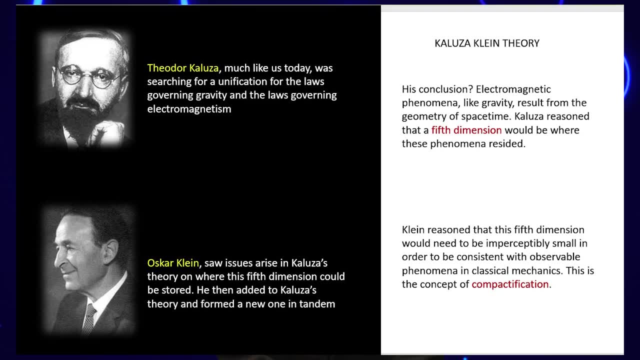 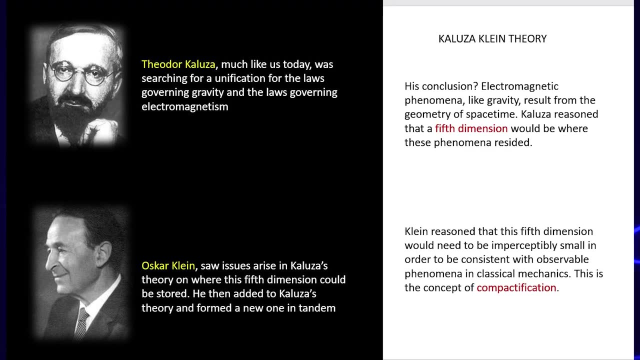 It's known not to be successful in what its original intent was to do. Namely, Kaluza and Klein intended to have a description of electromagnetism as sort of the fifth dimension, the dimension added to the three space dimensions and one time dimension. And some of those vestiges. 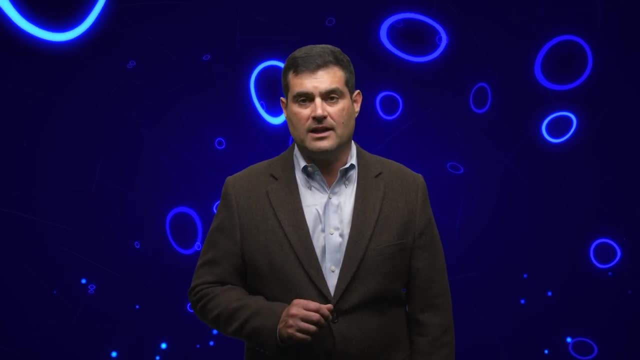 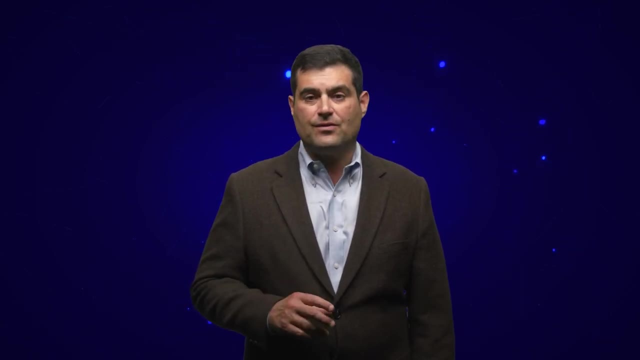 of that ancestor still remain and the theory of string theory is practiced today, So that model Kaluza-Klein theory was ruled out by observations that we make today, but it still provided a useful paradigm to assess the importance and perhaps the power that one gets when one adds an extra. 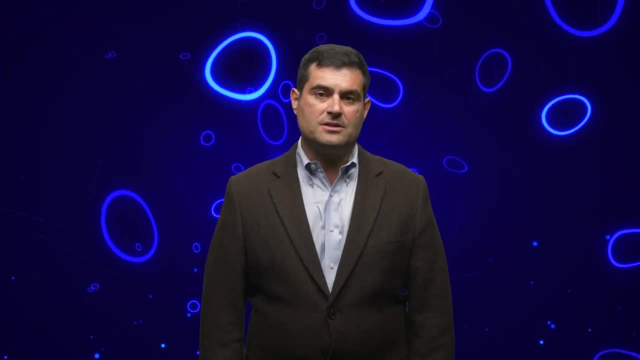 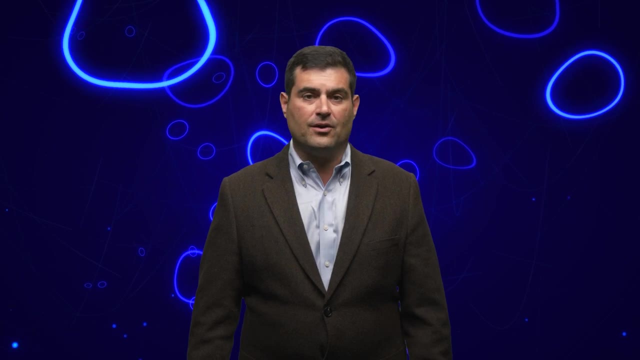 dimension. How can we reconcile the math of these extra dimensions and make things work out in the dimensions that we can test in the lab? Oftentimes, string theory gets criticized for being difficult, if not impossible, to test, and then it merely retrodicts rather than predicting. 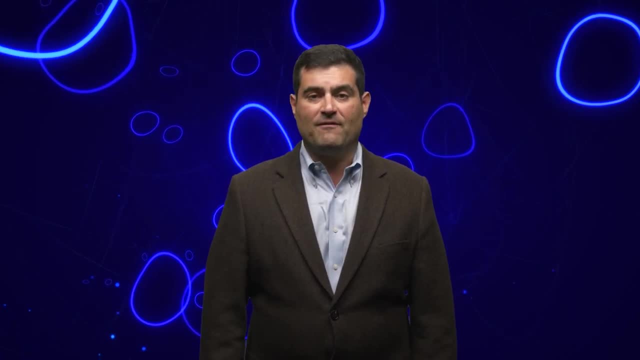 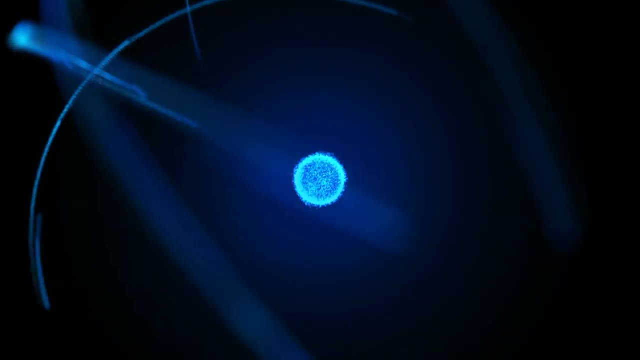 or conjecturing new phenomenon, which is what you'd like to do in a very, very powerful theory. Let's take a step back to the beginning. We're trying to combine general relativity with quantum mechanics. Now, matter at small scales will also have general relativistic effects. The question is: 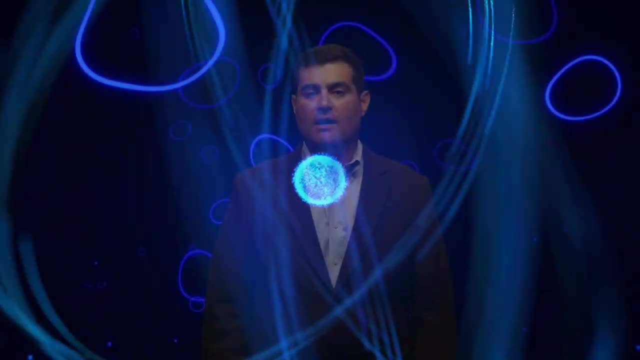 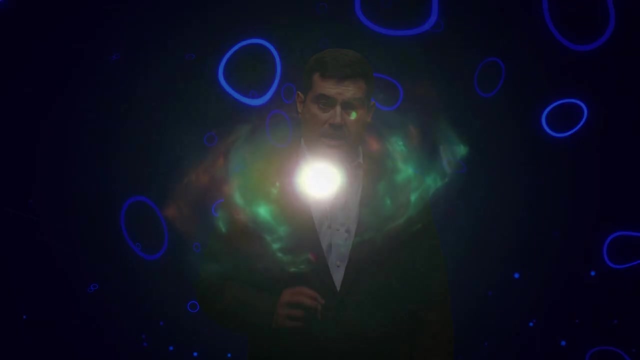 do we mandatorily need a quantum mechanical description of gravity at the smallest scales? We certainly don't need it for planets, We don't need it for galaxies et cetera. Those are more or less irrelevant. We may need it at the ultimate origin of time, if time began with. 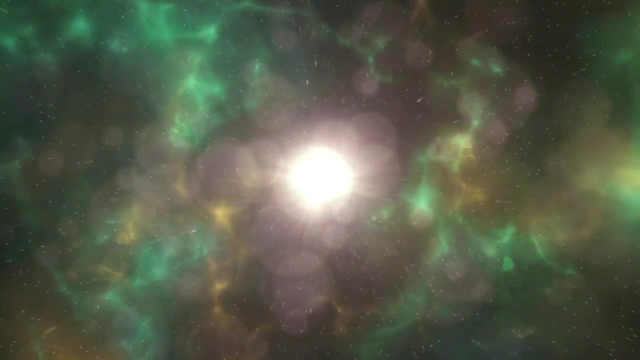 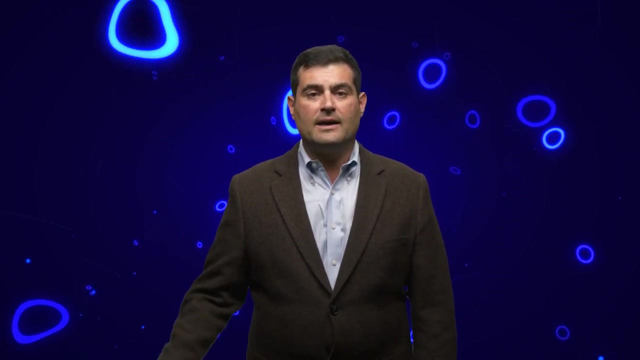 a singularity and also conjectures that eliminate the need for quantum, mechanical or singularity type events, namely the bouncing cosmological models that we considered in this video. I did about Ana Aegis and Paul Steinhardt's bouncing cosmological model, So we don't need them on the 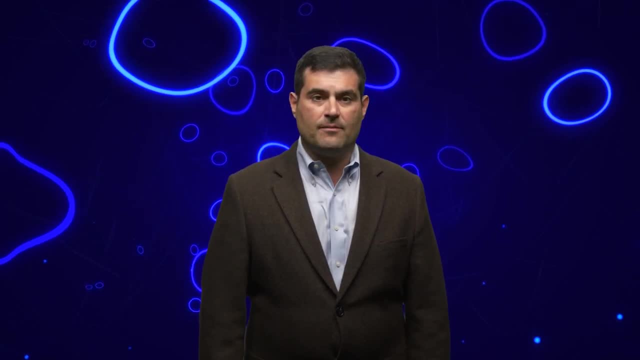 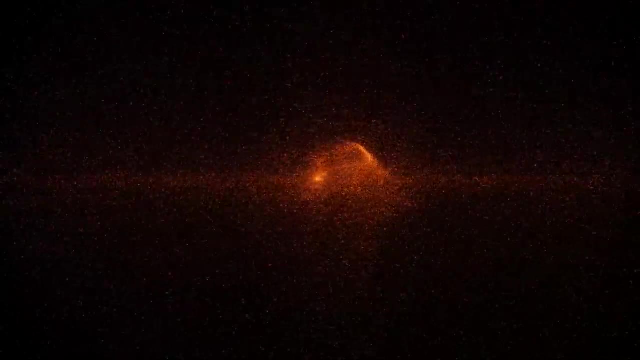 planet. The question is, how much can we do with the small scale information that we have? Gravity is dependent on space-time geometry, and quantum mechanics doesn't require necessarily the emergence of gravity in order to describe, say, the properties of the hydrogen atom. 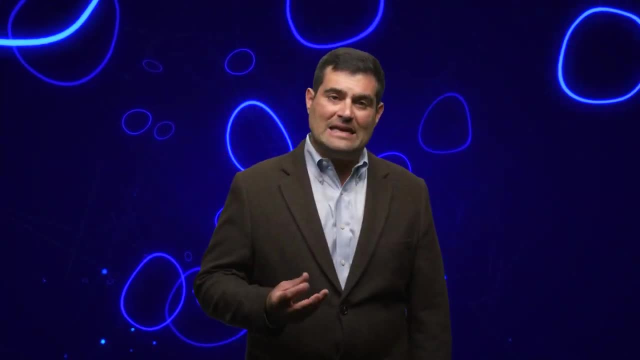 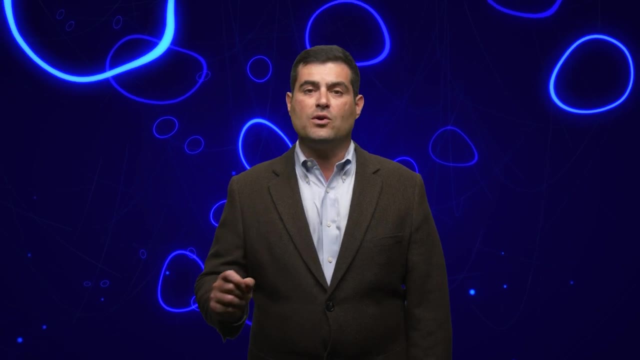 So it's a little bit tricky. We have to go to situations that we can't easily access in the laboratory. Nevertheless, it's a fair question as an experimentalist, as an assayer, to ask: could you have predicted new phenomena such as the two experiments that we've talked about? 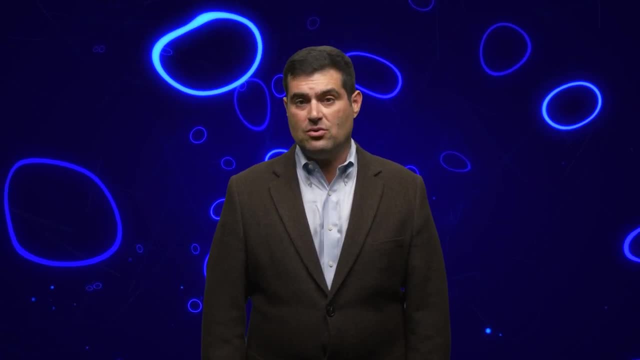 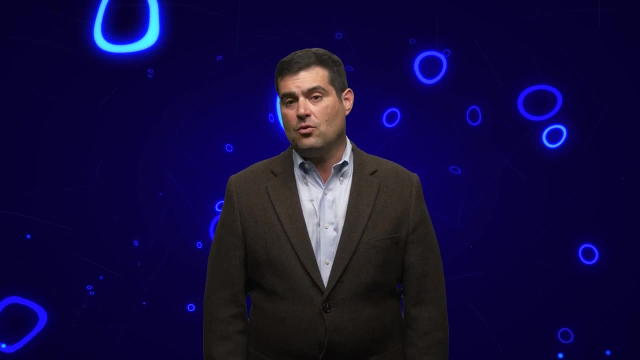 recently on the Into the Impossible podcast, namely the G-2 experiment about the anomalous magnetic moment of the muon, Put a link to that conversation that I had with Professor Dan Hooper and also with James Beauchamp, who we discussed the Large Hadron Beauty experiment, the results. 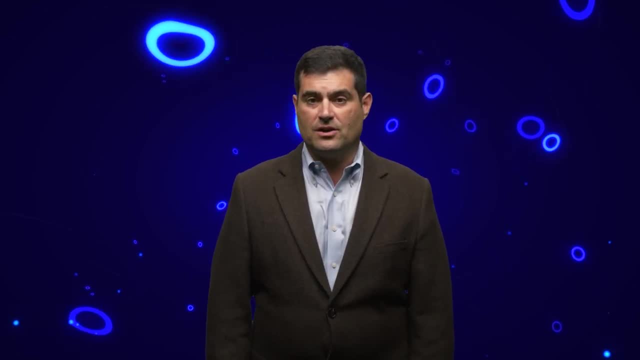 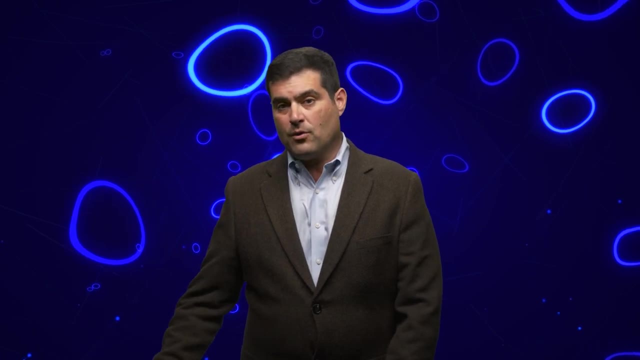 out of Geneva where we discussed the Large Hadron Collider's results back this spring. I'll put a link to that video over here. We had the conversation about the implications of that on a so-called fifth force and maybe whether or not these two experiments. 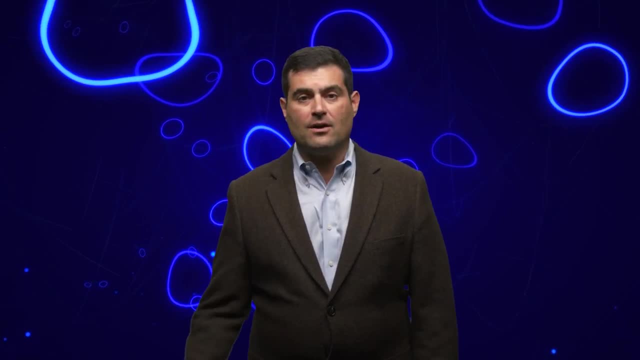 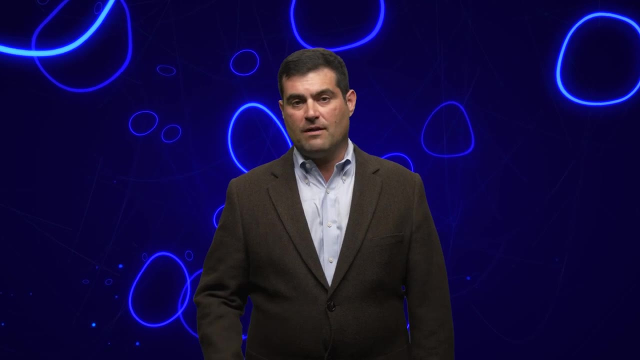 have been predicted by string theory. There are some, including Michio Kaku. in this conversation over here We talked about the God equation, his claim that string theory provides a manifest description of the theory of everything. He claimed that those actual experimental results. 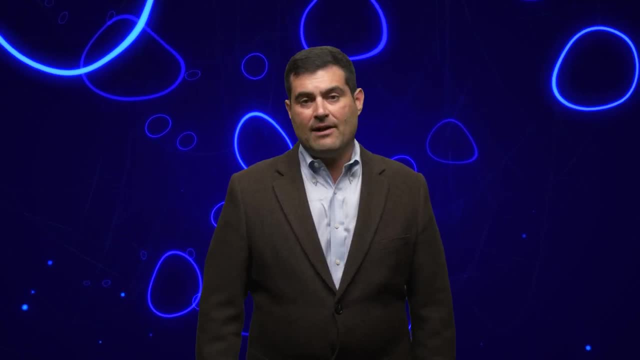 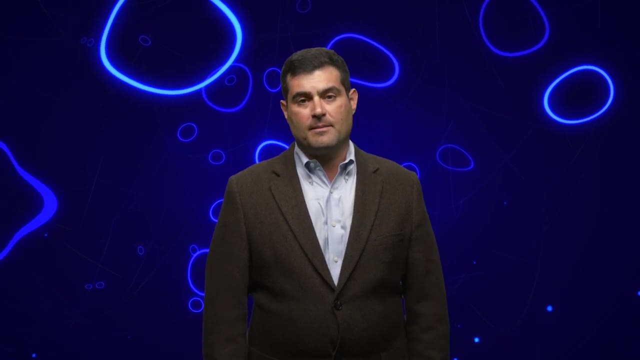 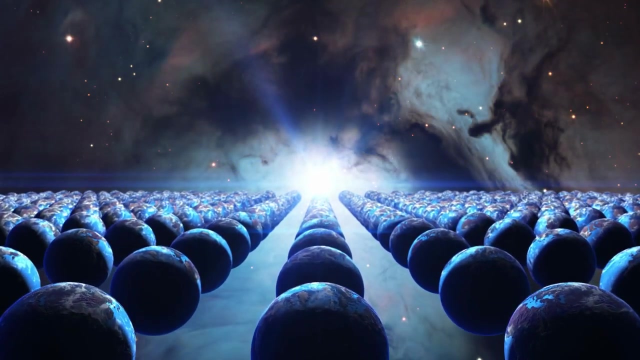 were contained in some sense in string theory's equations. I remain somewhat dubious and I ask you to watch this video and tell me if you agree, because the ultimate claim is that we, the experimental physicists, would have to come up with the vacuum state out of an infinite number of potential vacuum states for string theory. We'll talk about what. 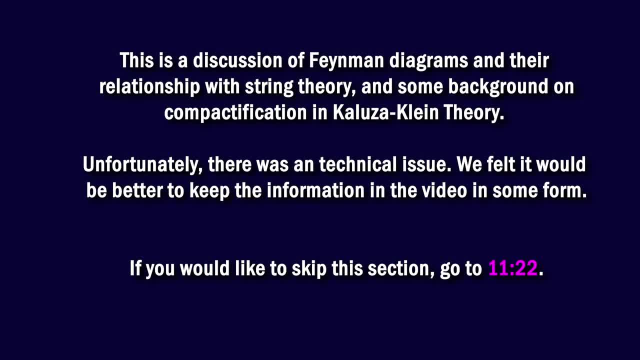 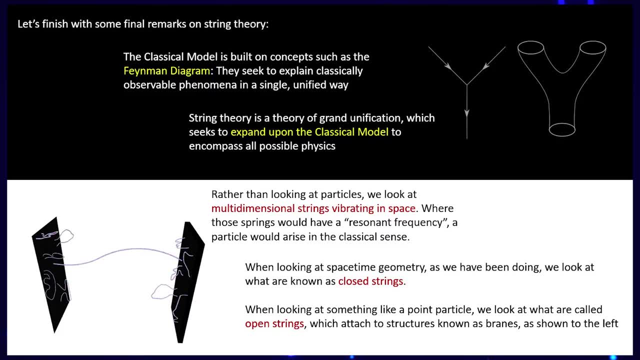 that means The standard model of quantum electrodynamics typically relies on these stick diagrams, often known as Feynman diagrams. Actually, they were invented by Richard Feynman, the renowned physicist of the 20th century. What string theory attempts to do is replace these. 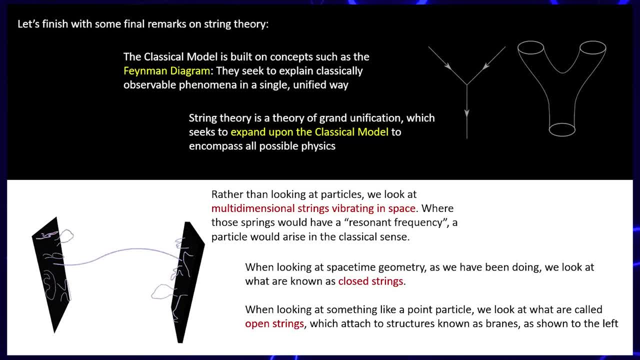 stick-like features with tubes or manifolds tracing out the world manifold, not just the world line of particles as they interact. So we can read the left version and translate to the right as follows: The left version describes two particles coming together, interacting. 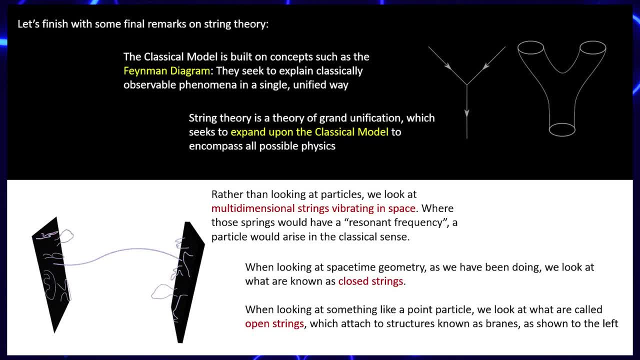 and a single particle emerging On the right. you have two closed loops, which are the simplest closed string, that come together and merge and out comes another string in the shape of another circular manifold. Those two different objects interact on the left as points at a single point. 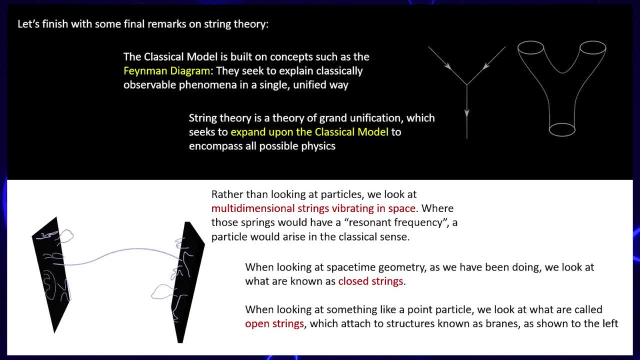 and you could see how you might get infinities arising. The point where they interact is of zero dimension. So if they have finite energy and finite charge, finite mass, et cetera, you could have infinite amounts a force, whether it be electromagnetic or 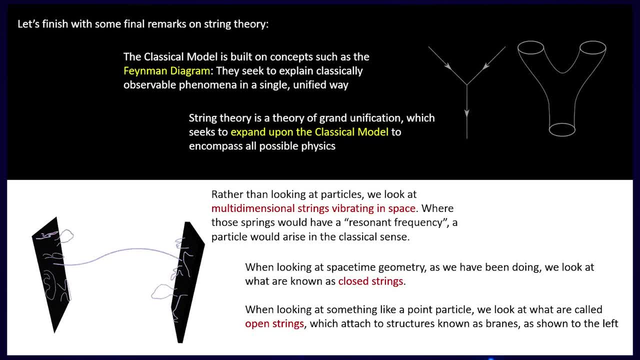 gravitational. if you just rely on the inverse-square law of separation, Alright. however, you have no such infinities. They come together and they join in a kind of mush together. They never go through a singularity or point-like rhobiologic divergence. So, rather than look at particles, 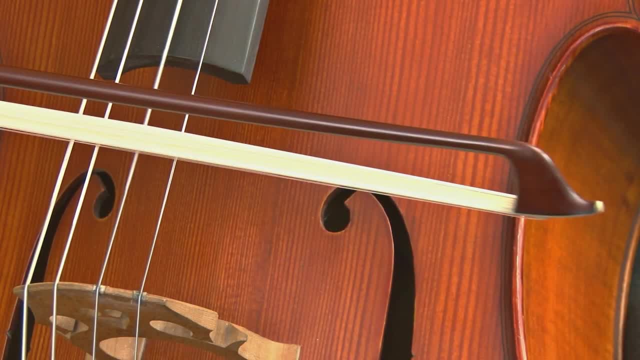 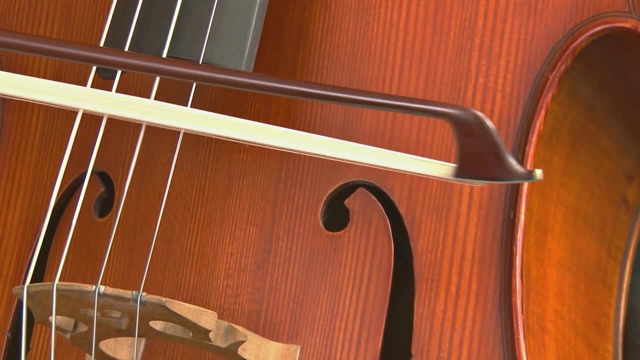 string theorists look at multi-dimensional strings of vibrating. in space, Where these strings would have a resonant frequency, a particle arises in the classical sense. When looking, Looking at spacetime geometry, as we have been doing, we look at what are known as closed. 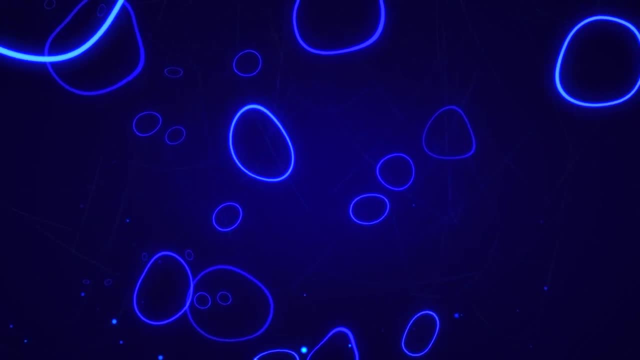 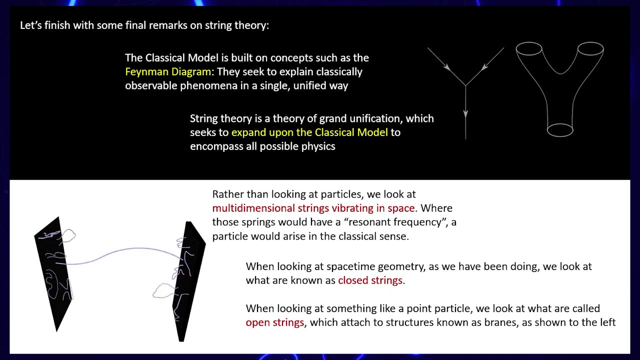 strings. When we look at something like a point particle, like a quark or an electron or a photon, we look at what are called open strings. These attach to structures known as brains, shown on the left. So we see that spacetime arises from string theory and we know that gravity is represented. 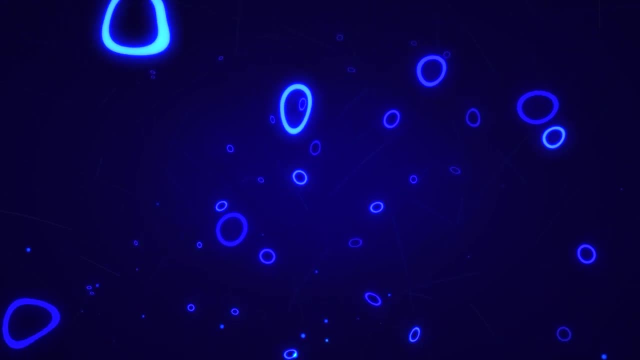 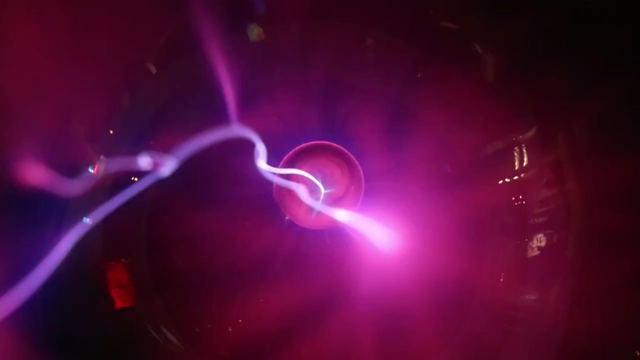 as a feature of curved four-dimensional spacetime. But if it emerges we would expect to see things like electromagnetism on an equal basis. So we can add to the 3 plus 1 dimensions of spacetime. we can add a fifth dimension. 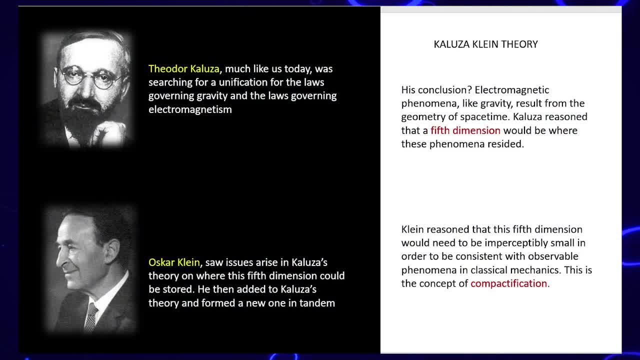 So Theodore Kaluza, much like what string theorists do today, is searching for a unification for the laws governing gravity and the laws governing electromagnetism. So the laws governing gravity will be the 3 plus 1 dimensions of general relativity. 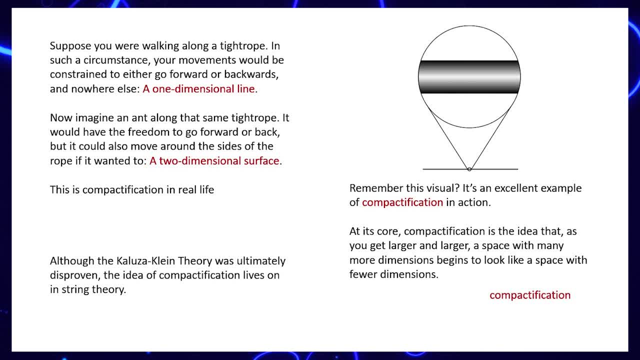 and the electromagnetic dimension will be an extra dimension And that he attempts to tack on, And what Oscar Klein did to it. he solved problems with Kaluza's original model where the fifth dimension could be effectively stored, And then he added to Kaluza's theory and actually formed a new version of it. 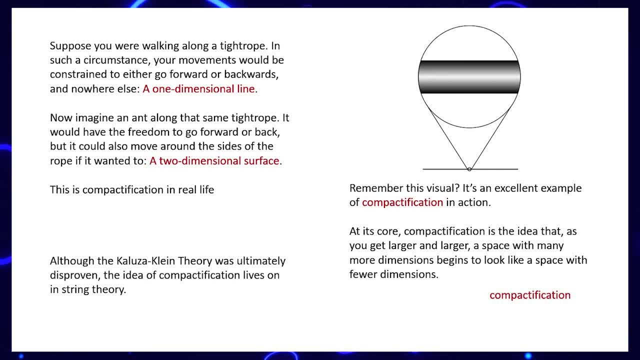 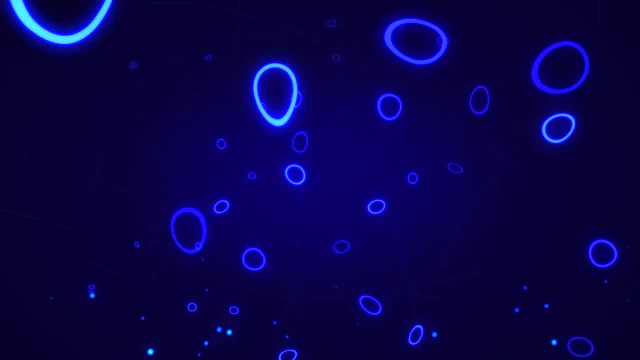 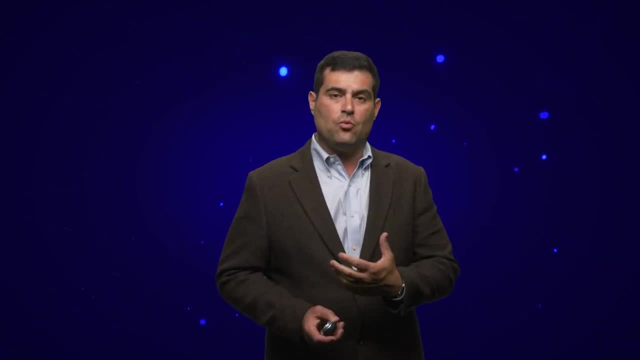 Electromagnetic phenomena, like gravity, would result from the geometry of spacetime. So Kaluza realized that a fifth dimension could be where the electromagnetic phenomena would be needed or where they would reside. But where does this fifth dimension reside? And there is something Kaluza used to hvorthere could have been a specific number of성. 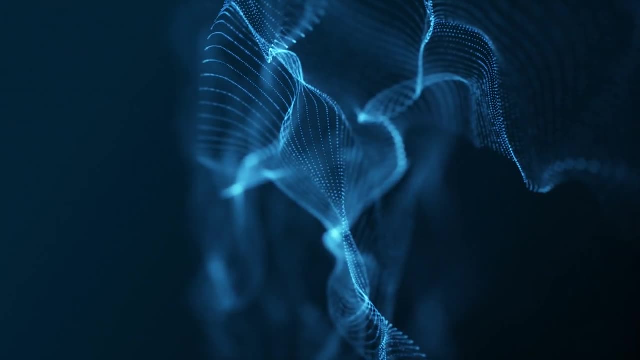 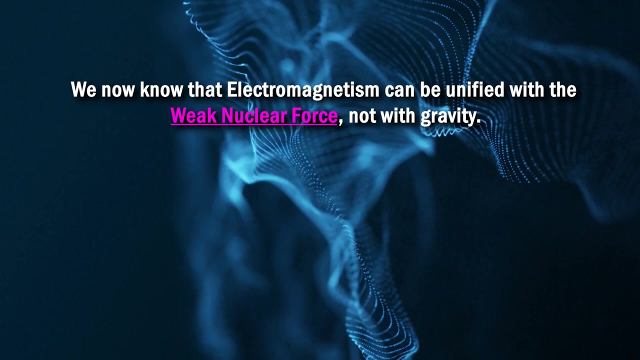 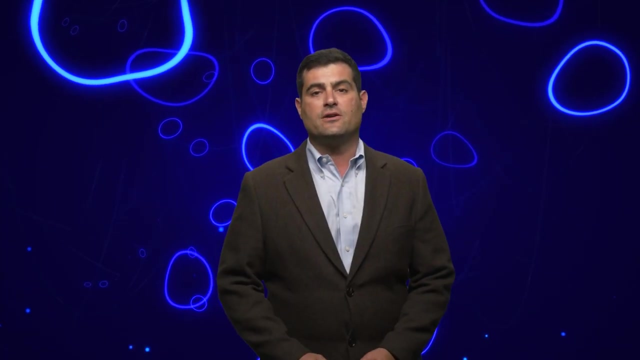 110 as a basic problem and insights to whatr string theorists do to this very day. He realized if the fifth dimension were supremely compactified into a microscopic, sufficiently small spaces, then you could getaround the problem of our not observing them, And then you could do all the operations, all the differential equations that are done. 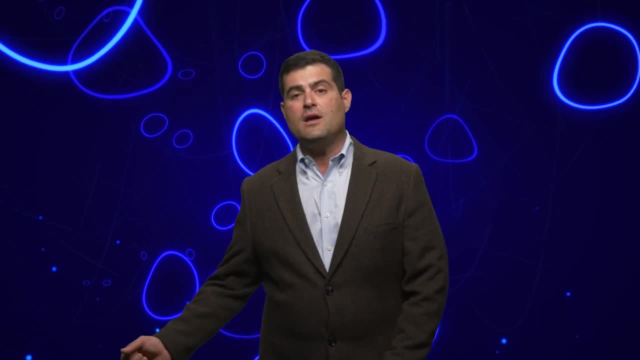 in general relativity effectively, and that would pop out a field theory for electromagnetism. Kaluza got an easy answer, but he couldn't come up with something right now. If you look through another copy of his dictionary you'll see that the записheed cha ADA was. 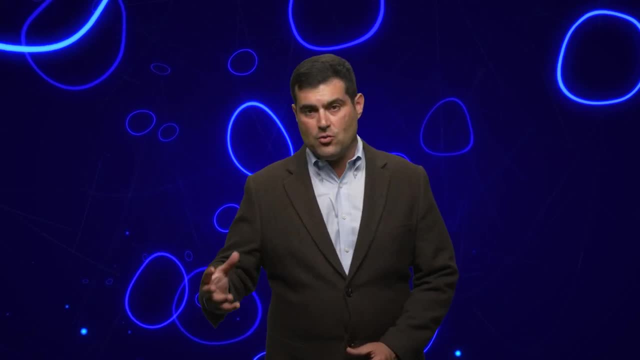 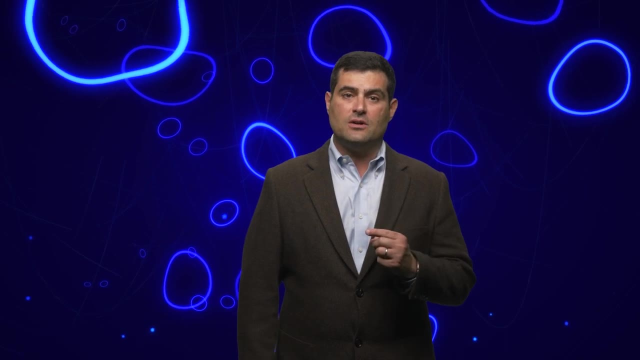 exactly the same. This gives a little bit more buffalo's point in terms of everyilah, If this is the right way now. his was the easiest five-dimensional manifold and you would get equations of Maxwell out, but you needed to do what was called compactification. Compactification is still central to our understanding of string. 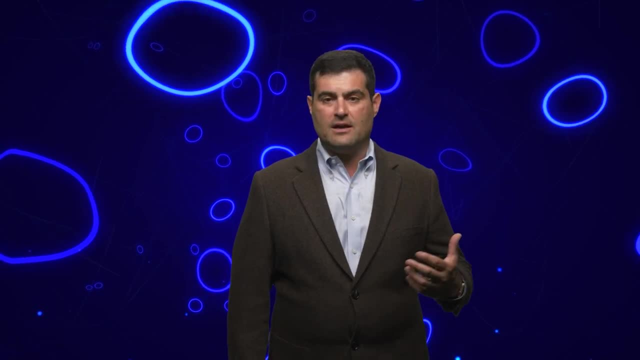 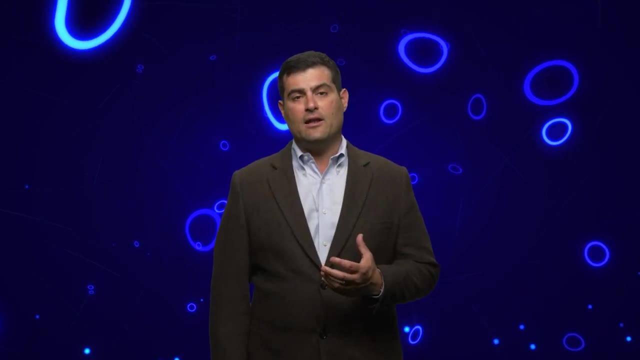 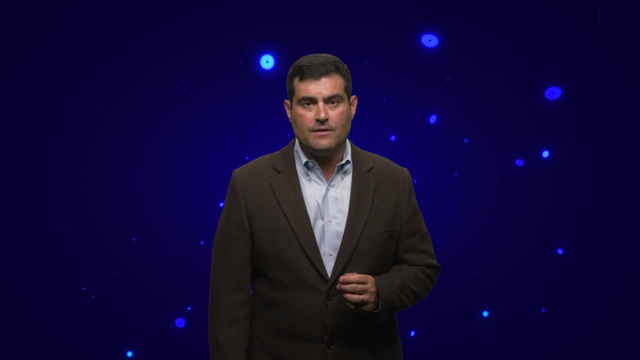 theory and perhaps to some reconciliation of the so-called grand unification of electromagnetism with the strong and weak nuclear forces. The fundamental element of string theory that allows for compactification and additional dimensions far beyond the three plus one dimensions that we know and love, is called the Calabi-Yau manifold. These beautiful, mesmerizing shapes would be. 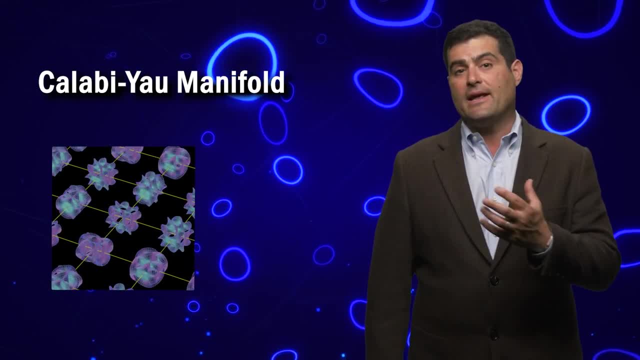 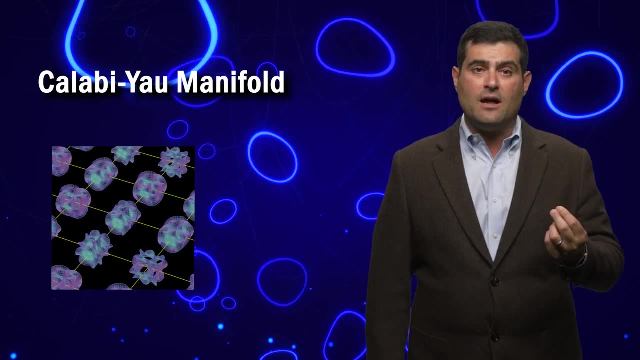 thought to be located at every point in three-dimensional space, operating at every moment in time, And you could add six or seven of these extra dimensions within a compactified manifold that you couldn't tell, because at our current scales we're still simply too far away. 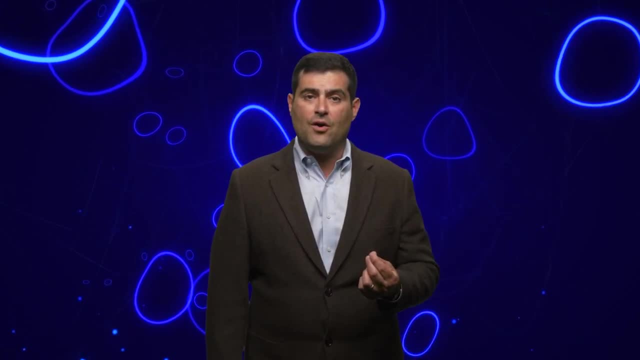 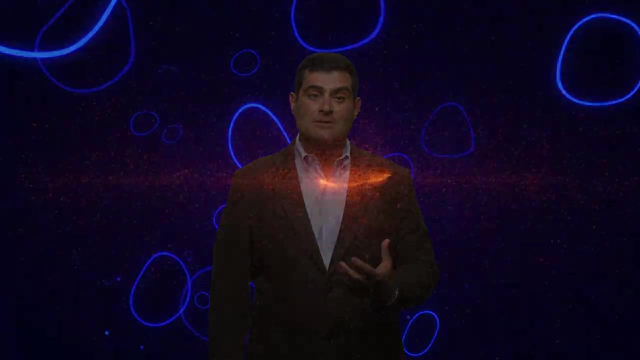 from them to perceive these things. These are really far below the size scale of the electron, which we can't even observe and shouldn't think about as a little tiny classical baseball anyway. And what allows it to incorporate gravity as well as the fermionic forces of matter that we are? 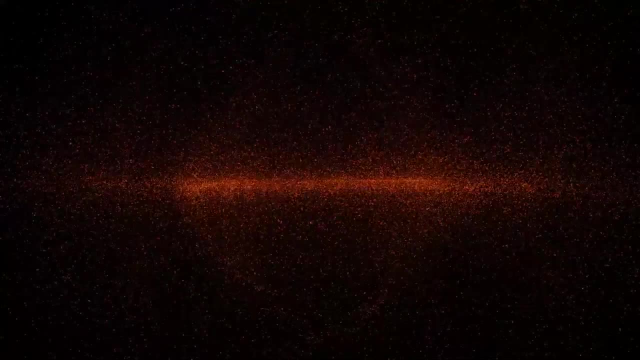 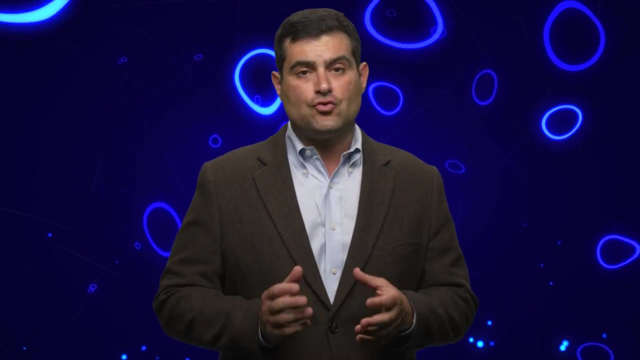 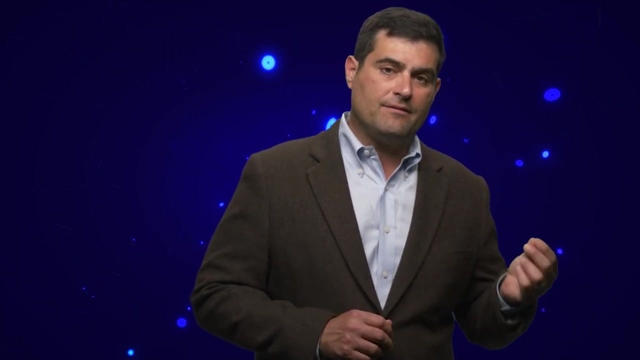 familiar with in the form of particles and forces and fields. So to an experimentalist, the situation is somewhat murky. We have predictions on a mathematical level that truly are intriguing. They represent a potential hope for physicists to unify the forces that operate on the very smallest scales with those that operate on the very largest scales. And yet, 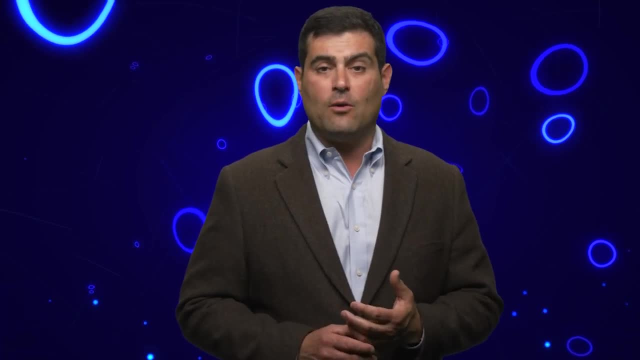 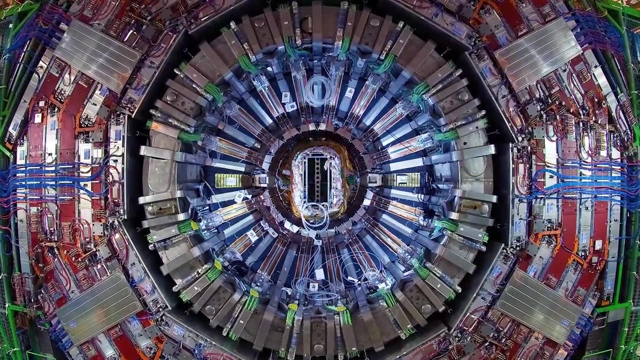 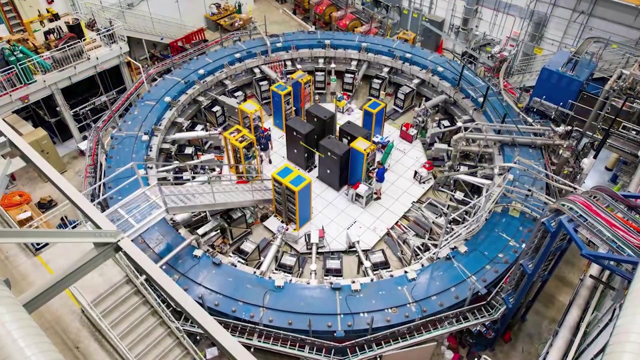 we fail to perceive, In other words, the observations at the Large Hadron Collider. when we talked about the LHCb experimental results in spring of 2021 with James Beecham and we talked about the G-2 results, those were not necessarily forecasted, predicted. They were more obtained when we look in the 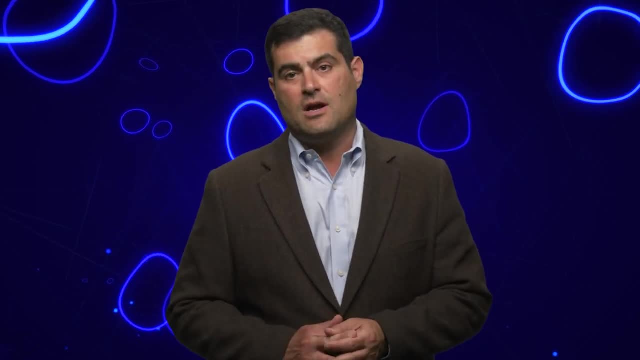 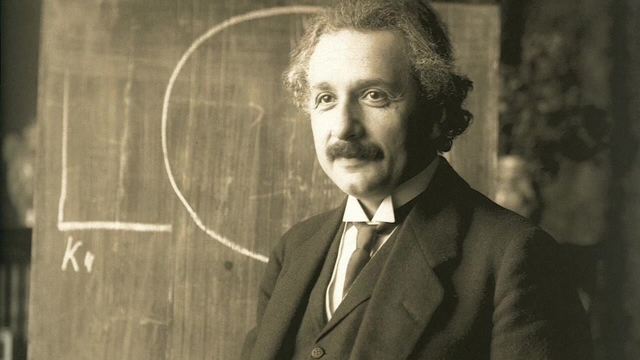 context of string theory by looking in what I would consider a retrodiction, And those are less satisfying. An analogy that I like to give is Albert Einstein's theory of general relativity. First, he could only make retrodictions to explain the, at that time, known behavior of the anomalies of 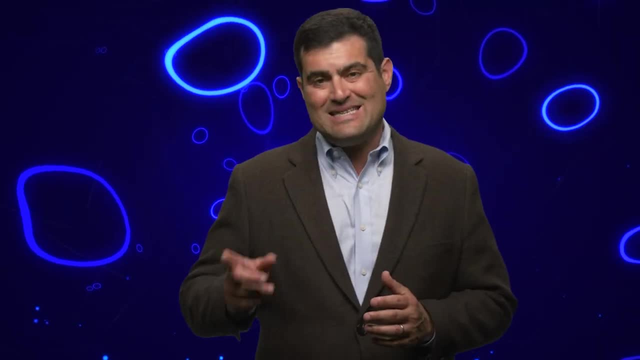 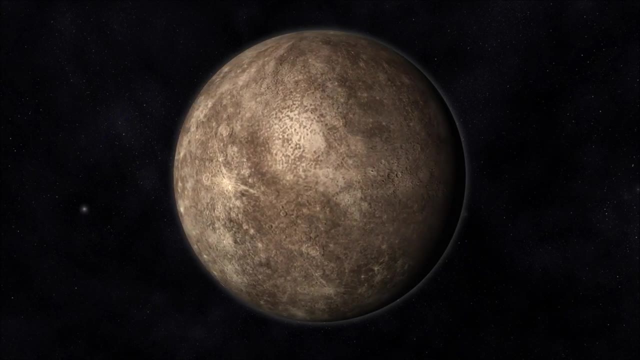 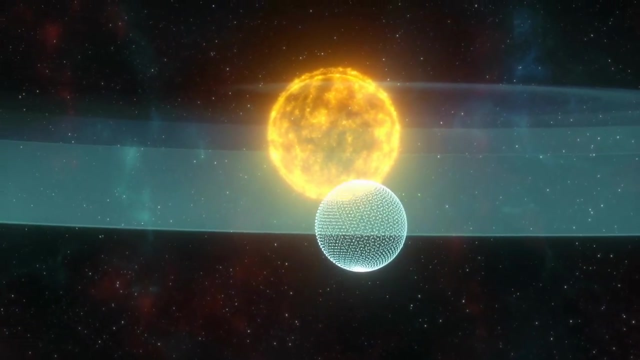 Mercury's orbit. So he knew that Mercury's orbit precessed anomalously And that was advancing its so-called perihelion advance, And that perihelion advance was impossible to reconcile with the laws of universal gravitation of Isaac Newton. And yet it was a retrodiction, It wasn't. 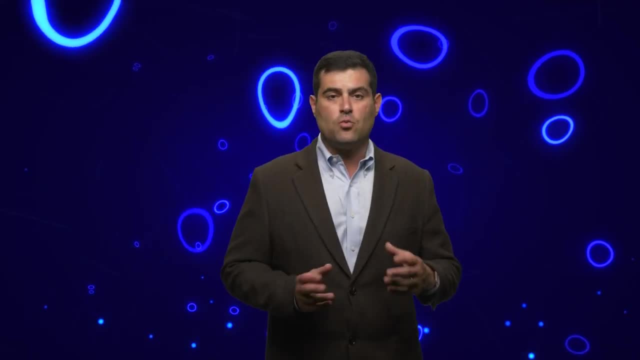 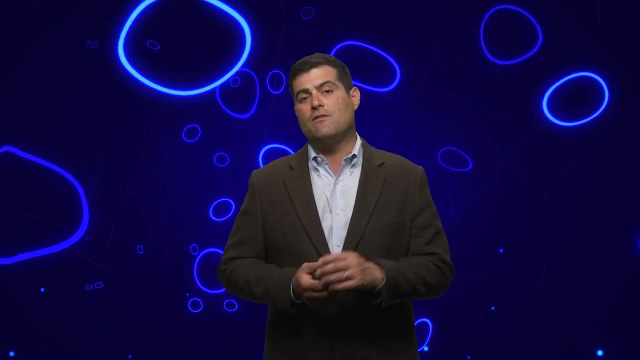 predicted by Einstein. It was explained by Einstein, And that was wonderful and magnificent. What's even more wonderful, more delightful, more delicious is if you make a new prediction, one that wouldn't have been expected a priori, And in that case, Einstein had a bounty of these. 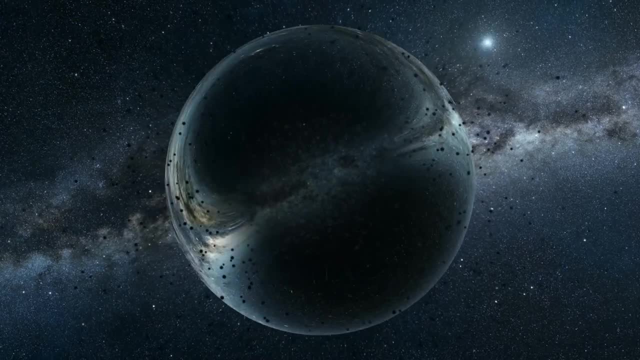 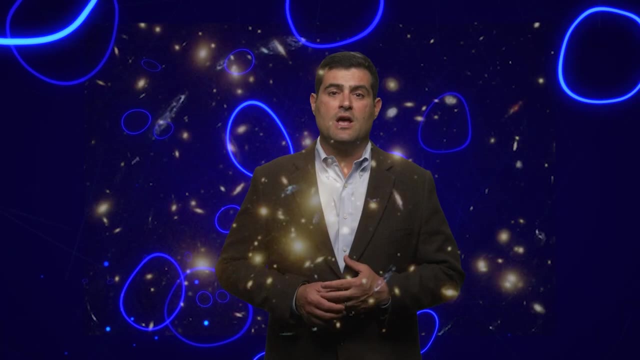 And one of them was the bending of starlight by massive objects like the sun, which is confirmed in the famous 1919 Eddington eclipse expedition. Another that wouldn't be confirmed for many more years was strong gravitational lensing, the Shapiro time delays and also the existence of 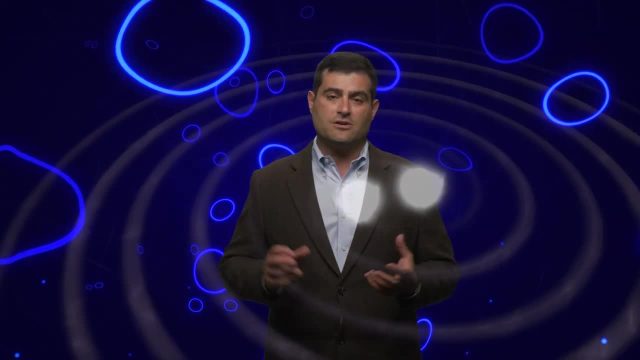 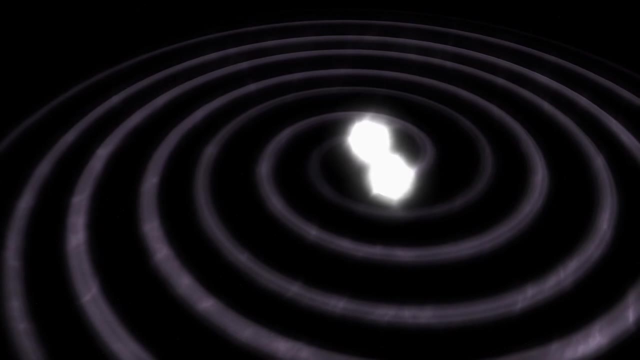 gravity from the orbit of massive objects known as black holes or neutron stars, compact objects moving very close at relativistic speeds and finally coalescing together, producing enormous showers of gravitational wave energy. Those are predictions of the theory of relativity. What 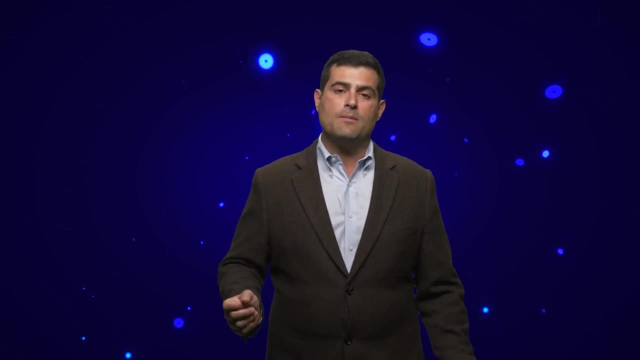 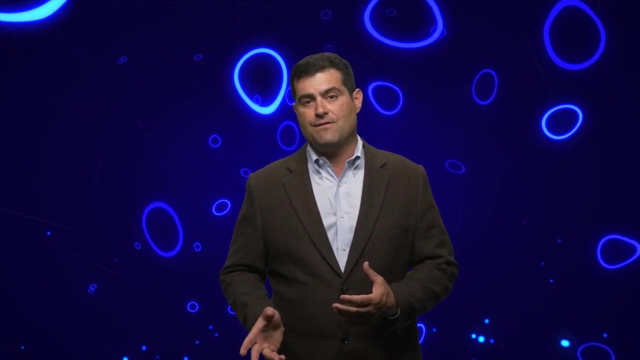 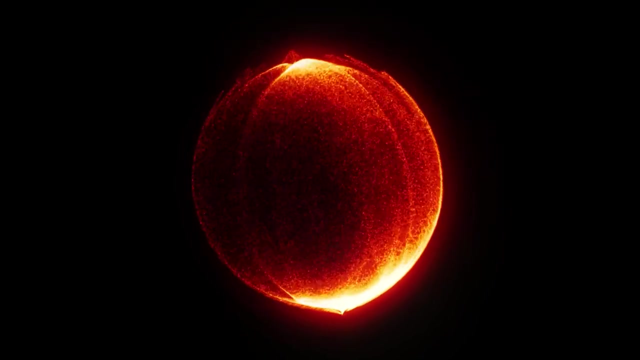 predictions are there in the string theory landscape? What can we predict that we would not have known about and can be surprised about? It would be wonderful to explain existing phenomena, such as the sizes and forces and fields and coupling constants and particle masses, etc. That would be great. We already know them, We've measured them, We'd 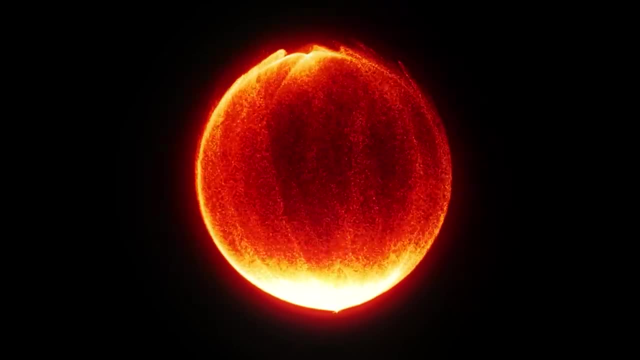 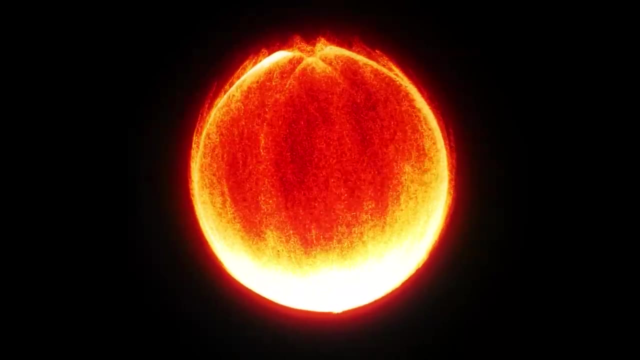 like to have a theory, maybe that predicts them or retrodicts them rather. But it would be very cool if the string theory formalism could predict a new phenomenon. that would fit in beautifully in the framework of string theory, And for now we have to wait for that. there would be virtue in looking 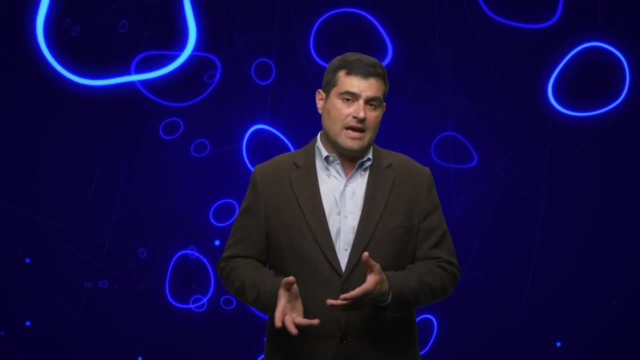 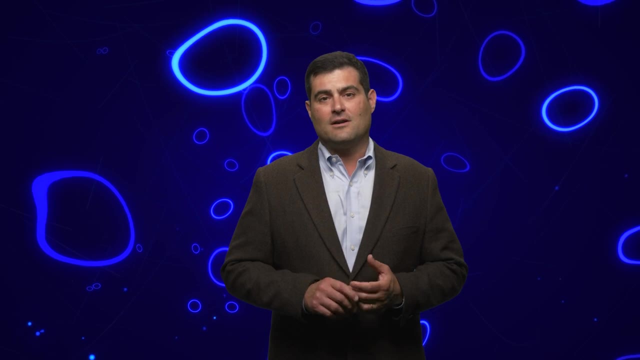 at maybe low energy limits of string theoretic predictions to see if there is data that are lurking in existing experiments or near term experiments. So thank you for joining me in this sub episode entitled string theory for experimentalist as part of the assayer project to understand and to test. 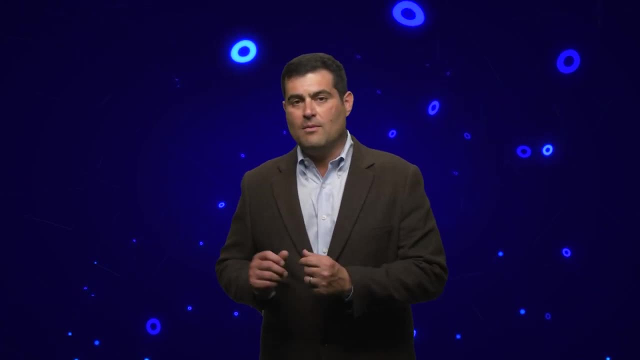 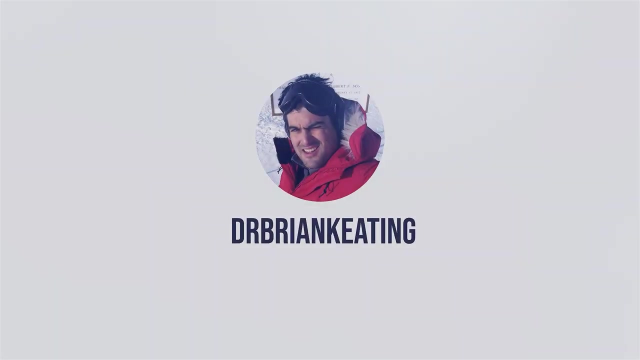 and compare against existing data with new models and see what comes off the stone. Thank you so much for going into the impossible with me. I'm Brian Keating, Chancellor's Distinguished Professor of Physics and co director of the Arthur C Clarke Center for Human Imagination. Thanking you for watching this episode of into the impossible.